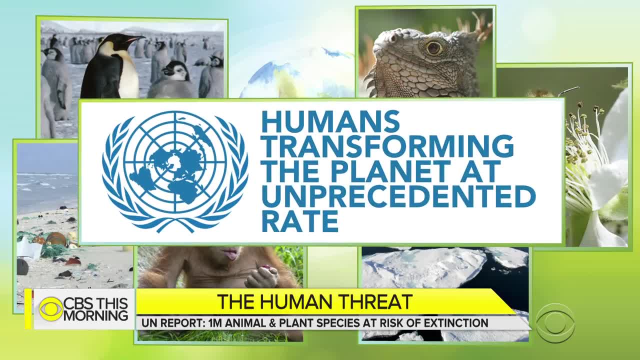 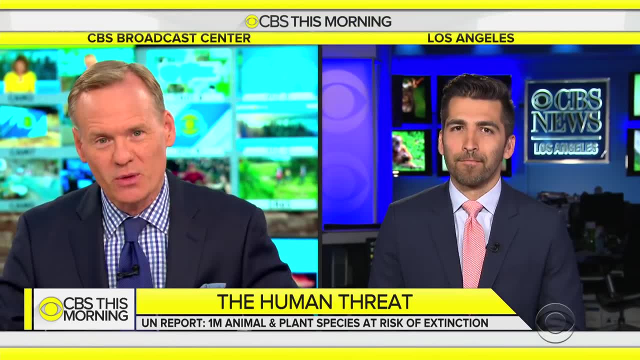 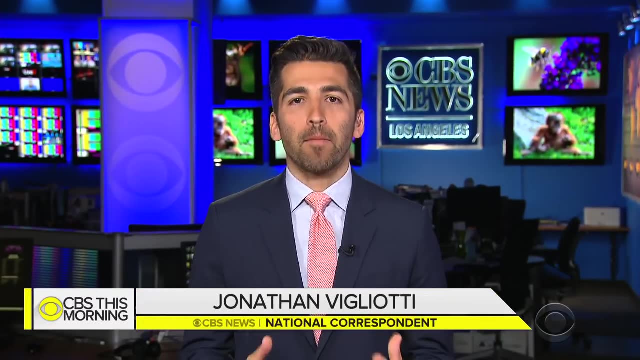 warning: Humans are transforming the planet's natural habitat at an unprecedented rate. Jonathan Vigliotti is in Los Angeles with what the future could look like if nothing's done. Jonathan, good morning And good morning John. Scientists say the report is a landmark in the 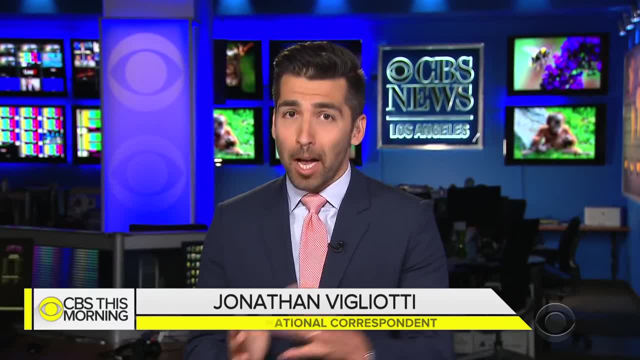 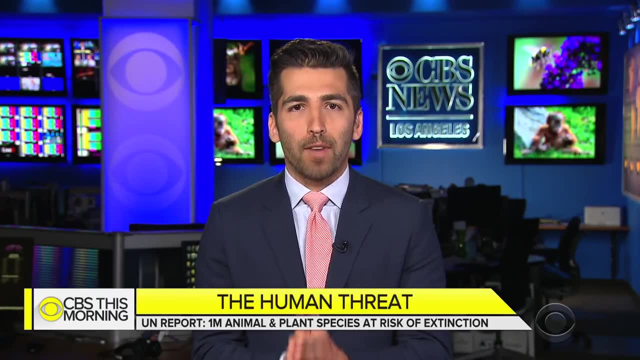 conservation battle. Not only was it compiled by scientists- hundreds of them- it was approved by diplomats as well, from 132 countries, including here in the US. They say human survival depends on healthy animals and plants, and destroying them ultimately hurts us. 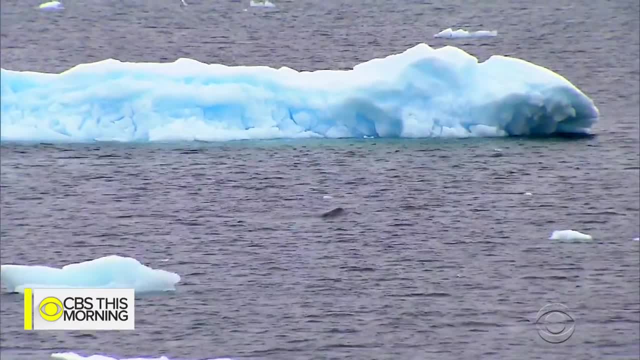 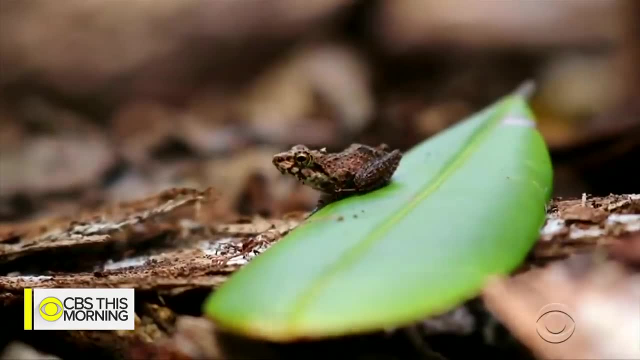 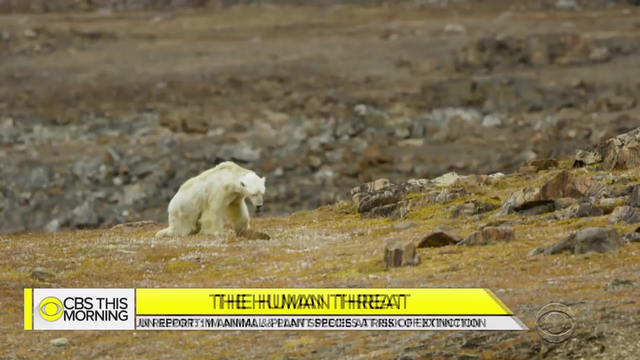 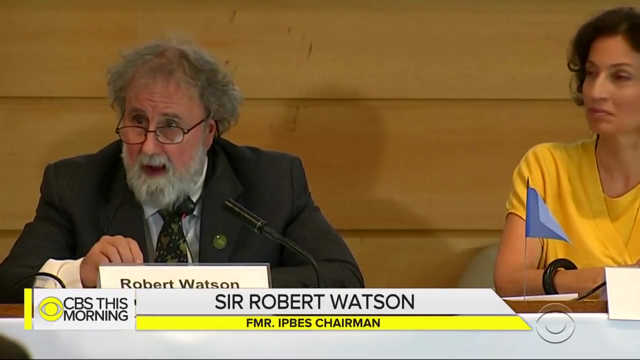 From penguins and killer whales in Antarctica to orangutans in Indonesia and sea turtles on the Great Barrier Reef. animals all over the world find their habitat threatened by human activities like unsustainable farming and pollution, and their very survival is at stake. Biodiversity is important for human well-being and we humans are destroying it. 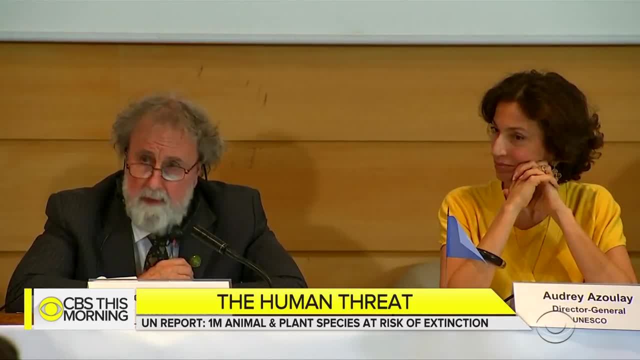 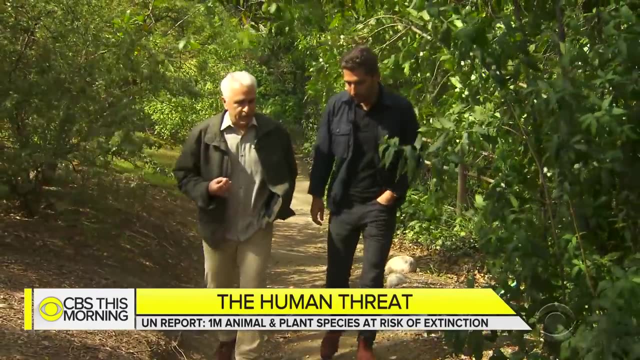 Although it was notable for being comprehensive, the report's specifics came as no surprise to some. We're looking at a crisis. I mean we're really. this is code red. Dr Thomas Smith is with the UCLA Institute of Environment and Sustainability. 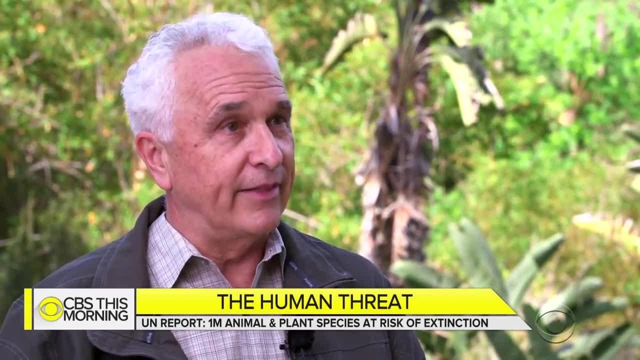 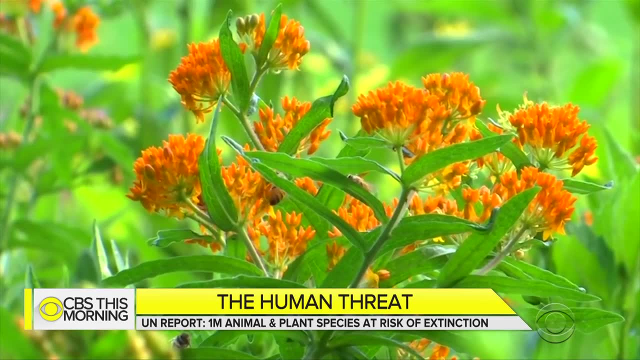 Biodiversity is basically all the living parts of the planet, and that includes us. So we depend on animals and plants for our food, for our pollinators. If we lose those elements, we're losing essentially the resources that humans use to survive. 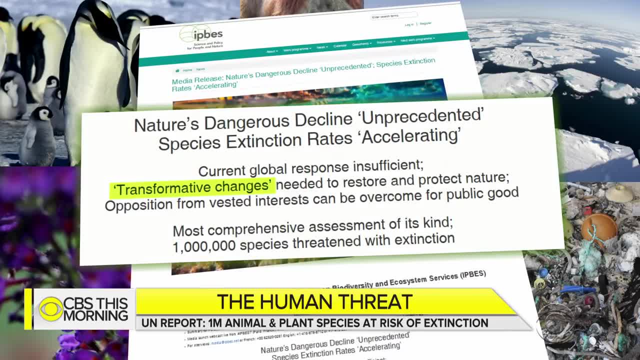 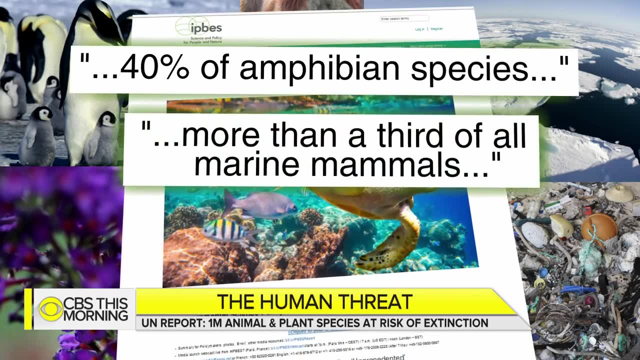 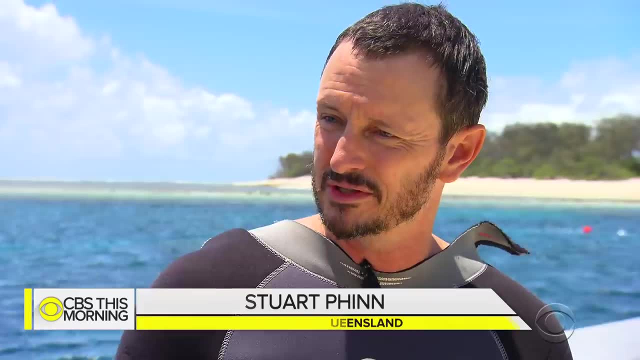 Unless society makes what it calls transformative changes. the report predicts that in the next few decades, more than 40 percent of amphibian species could go extinct, along with over one-third of marine mammals and more than one-third of the world's coral reefs that give them life. People depend on the fish stocks that come out of that, for 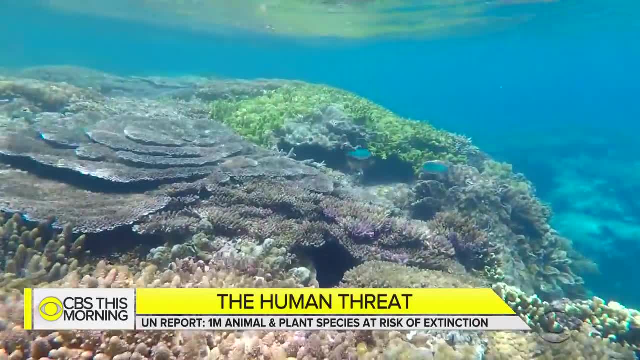 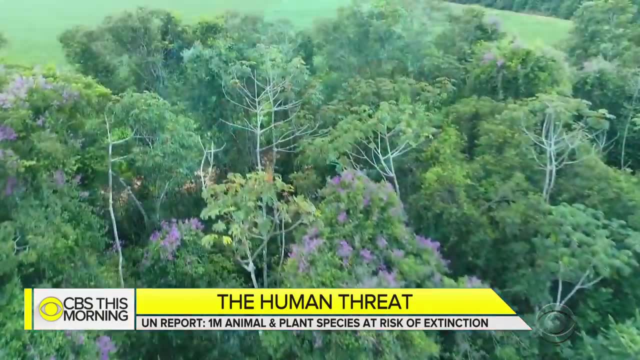 subsistence. CBS News has circled the planet to show how loss of animals and plants can impact human populations: from the waters off Australia to the Brazilian Amazon, which creates weather systems that cool the world, These forests, the world's a much hotter and drier place. 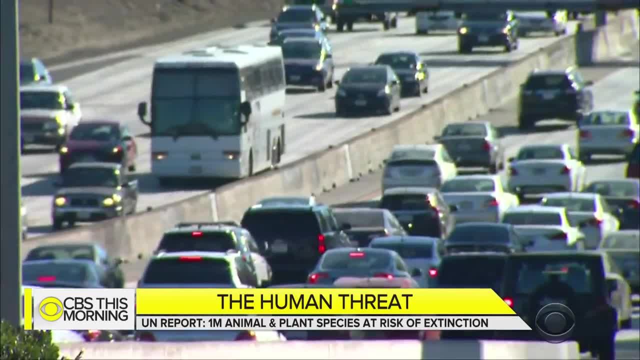 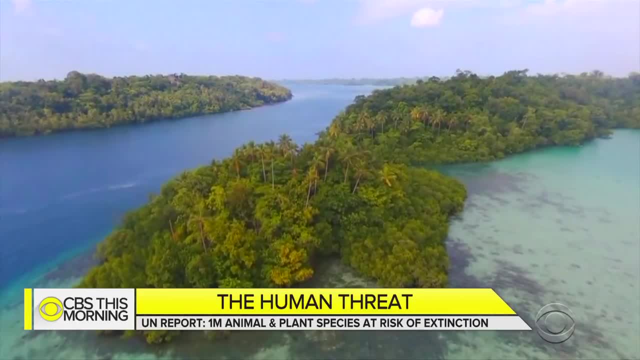 Scientists note that more than seven billion people on this planet depend on the delicate balance of biodiversity to survive, And while the human population is growing, the Earth's resources are not. If action is taken now can this be reversed on a large scale.